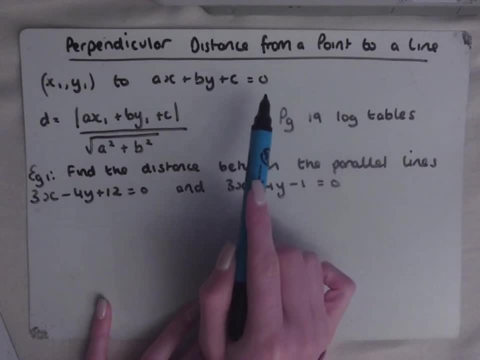 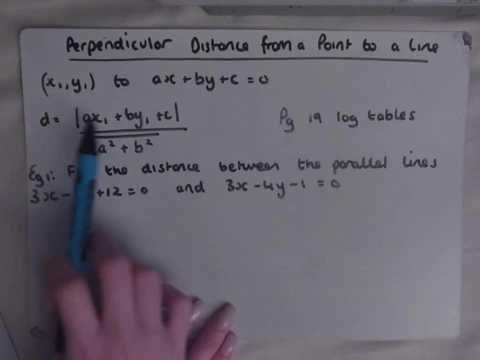 So it needs to be in this form. So if you're given any other type of equation, you need to make it: ax plus by plus c equals 0. So the perpendicular distance d is again the absolute value of ax1 plus by1 plus c over the square root of a squared plus b squared. 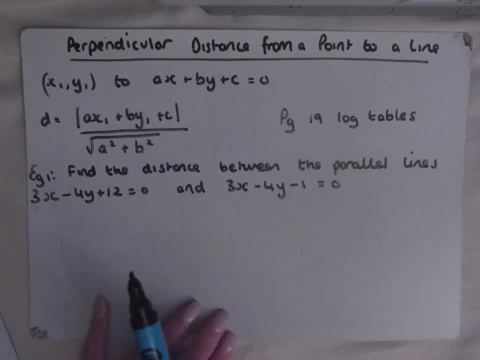 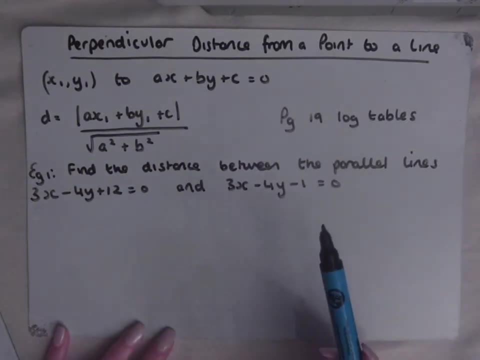 So, whatever the top line is, you're going to take the positive value of it. So find the distance between two parallel lines. You have these two here. Now to find the distance, you're getting the perpendicular distance from a point on this line to this line, or a point on this line to this line. 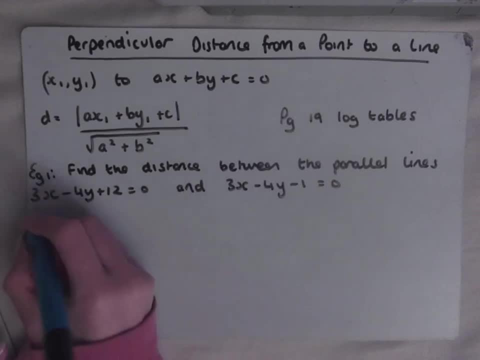 So we're just going to find any point on this line. So what we'll do is we'll let x equal 0, and we'll get minus 4y is minus 12, so y is 3.. So we have a point: 0, 3, okay, and we have this equation here. 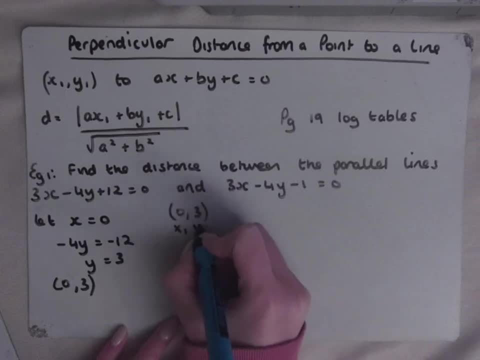 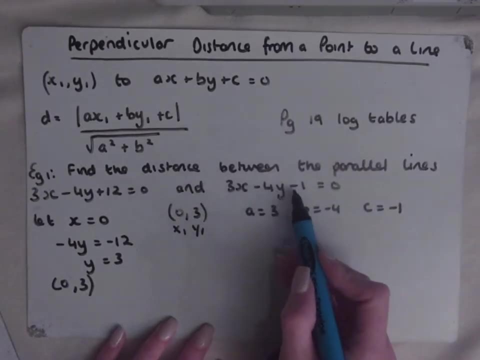 So 0, 3 is our x1, y1, a is 3, b is minus 4, and c is minus 1, okay, ax plus by plus c, And we're just going to fill it into our formula. 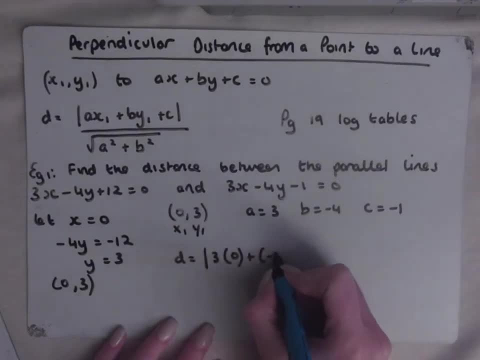 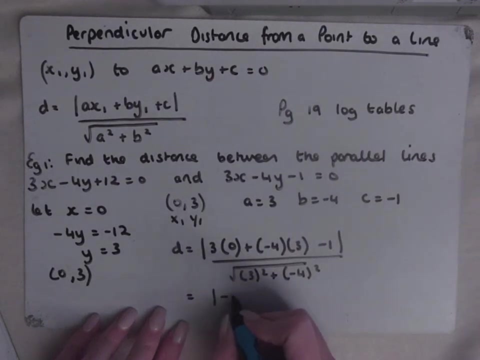 So ax1 plus plus by1 plus c, all over the square root of a squared plus b squared, okay. So what we get is minus 12 minus 1, which is minus 13 over, and this is 9 plus 16 square root of 25,, which is 5, okay. 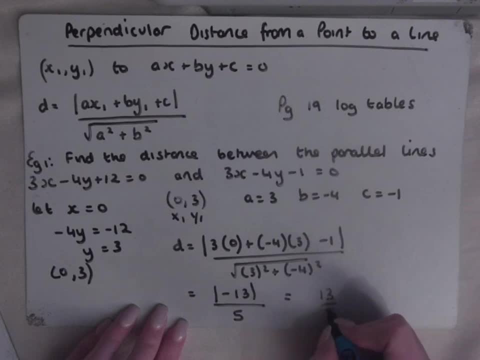 Now we're taking the absolute value, so that just becomes 13 over 5.. So the distance is 13 over 5 units. All right, That's it, everybody. Go ahead and take it off. All right, We're just going to find our point. So the distance is 13 over 5.. So around here, this one, what we're going to do is we're going to subtract parents, So you know, will show a plant right, And what they're saying is that one, two, three, five. Okay, Do that over 15 times. Do that over 15 times. We know you can do. And what you're going to do is if you're taking out 1, 3 via 1, 2, 3, and 5, and you're not being able to subtract that number from 1, 3,. OK, So you're going to get 1 over 5 by taking out 1.. So that's it. 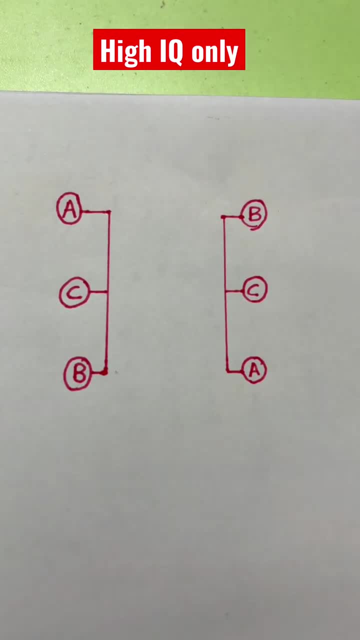 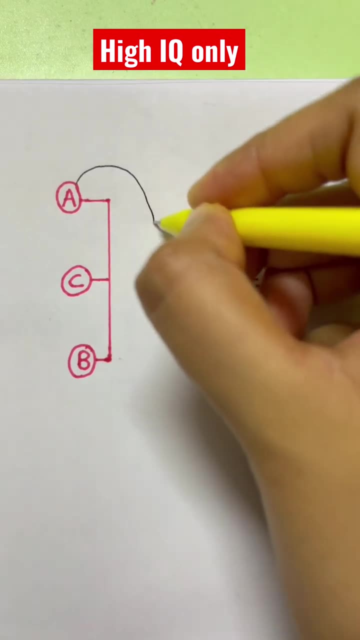 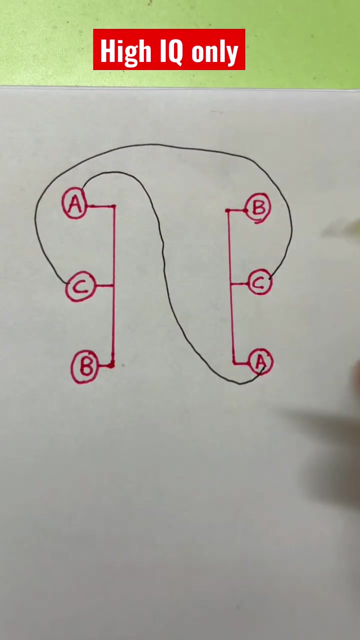 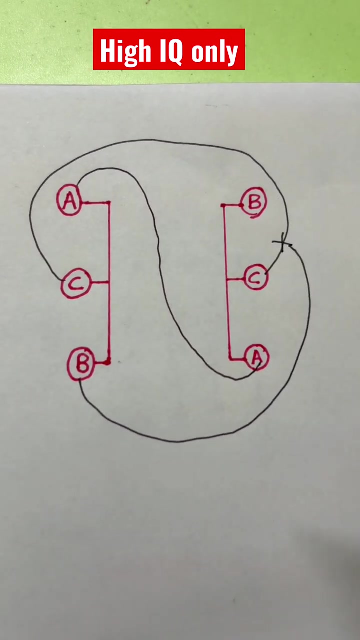 If your IQ is more than 150, you can easily solve this question. All you have to do is just join the circles from A to A. I'll just demonstrate from A to A. and likewise you have to do from B to B and C to C. So it's from C to C and same way from B to B. Oh no, but you cannot cross the lines. So this is what makes it difficult. So if you know the answer, do this video.